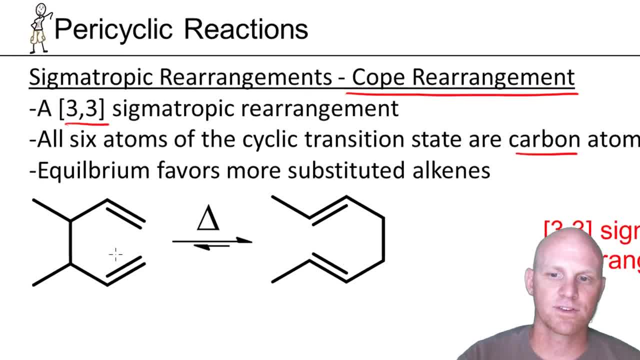 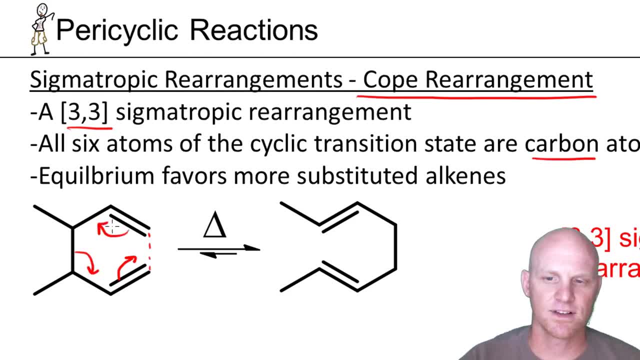 they're all carbons, and that's what makes it a Cope rearrangement. If we kind of follow the movement of electrons here, we're going to form a new sigma bond right here. so and again, cyclic movement of electrons. everybody gains and loses a bond. There's the 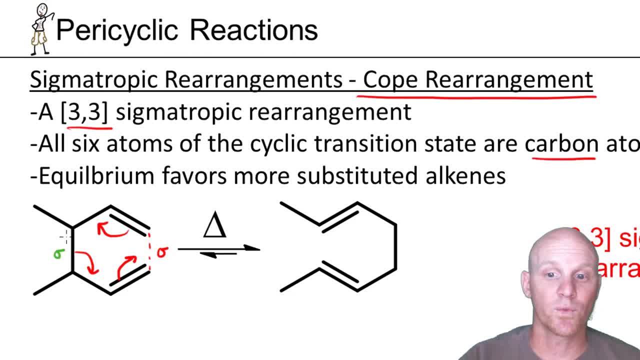 new bond we are forming, There's the old one we're breaking. So the old one we're breaking is between these carbons. The new one that we're forming is between these carbons and if we count on this side, 1,, 2, 3, from where we're forming to where we're breaking is three atoms. and on this, 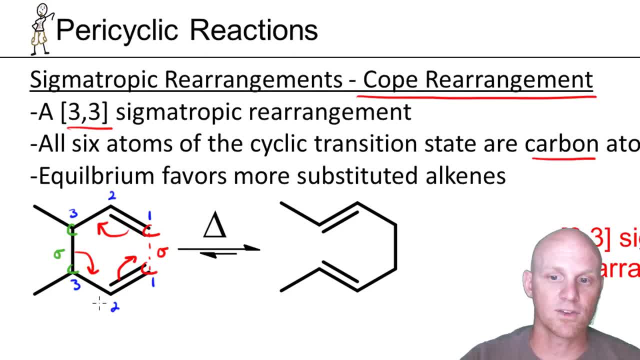 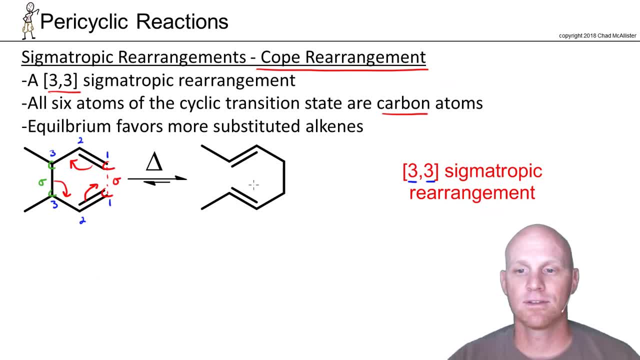 side 1,, 2,, 3, from where we're forming to where we're breaking three atoms. That's what makes it a 3,3-sigmatropic rearrangement. So, and usually it's just pure alkene stability that you know. 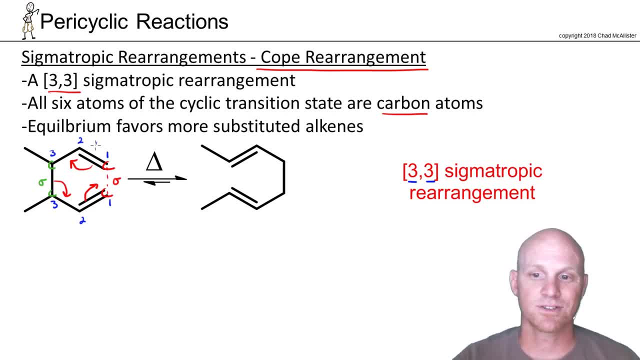 drives the equilibrium in this case. So if we look at our alkenes here, this one here is just mono-substituted alkene. This one's also just a mono-substituted alkene, but on this side this one's di and this one's di and the more substituted alkenes are more stable. 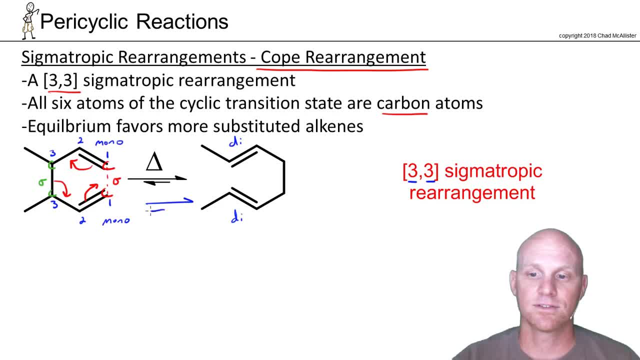 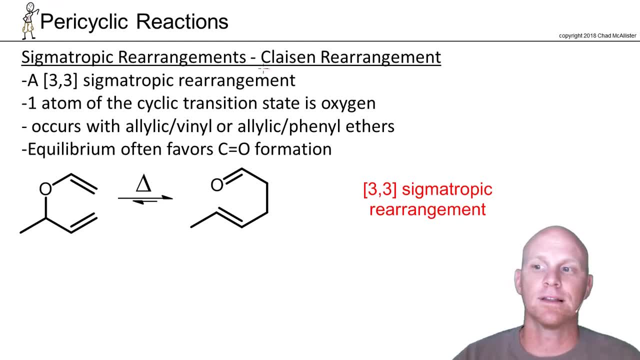 and that's why the equilibrium here is definitely shifted to the right, and it'll favor formation of the products in this case. So now we'll deal with the Claisen rearrangement. and the Claisen rearrangement, as we said earlier, is also a 3,3-sigmatropic rearrangement. 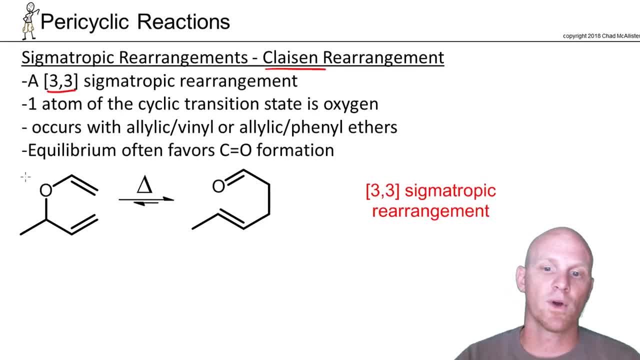 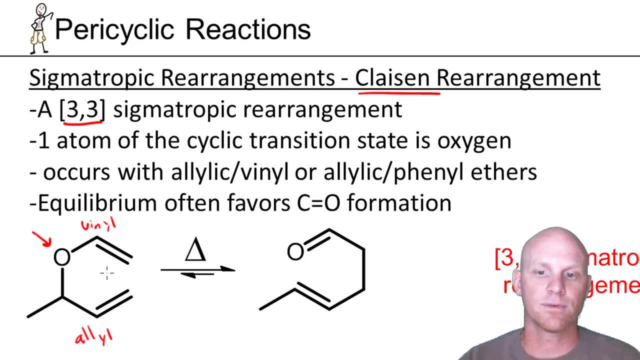 just like the Cope was. but the big difference here is you're going to have an oxygen being one of them and generally you're going to have like a vinyl allyl system here. so notice ether- I should say specifically So- and in this case your vinyl allyl ether definitely. 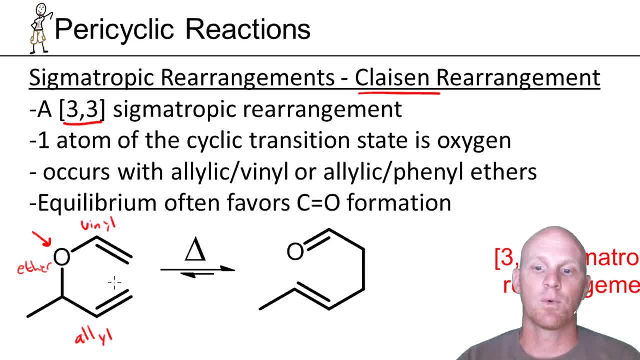 subject to the Claisen rearrangement. It's just thermal condition reaction here and we're going to have a cyclic movement of electrons again. so maybe I will form a bond right here, break this one and form a bond right here and then form a new sigma bond right here. 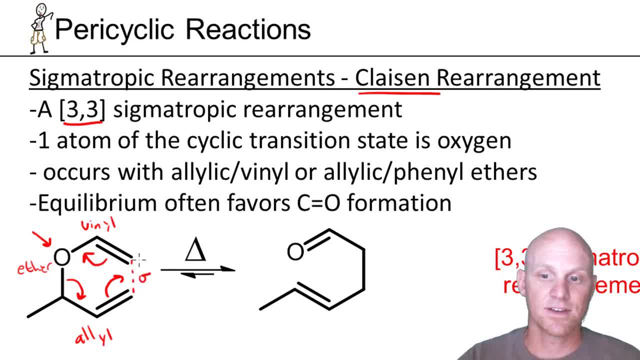 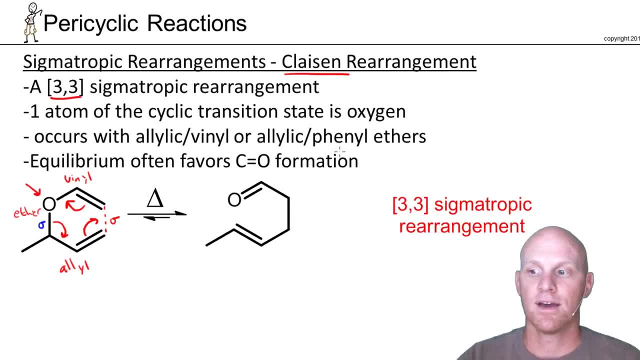 So I'm forming a new sigma bond right there in this position, I am breaking one right over here in this position, and one, two, three, one, two, three. hence it's a 3,3-sigmatropic rearrangement. 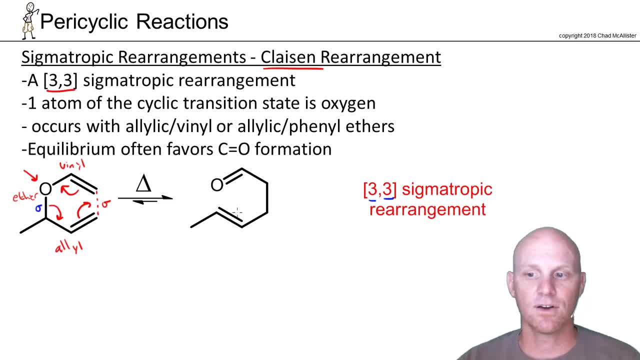 So, and in this case we're going to end up with a double bond oxygen here and an alkene here- and a carbon oxygen double bond is more stable than a carbon-carbon double bond, If you recall. that's why in ketoenol tautomerase, 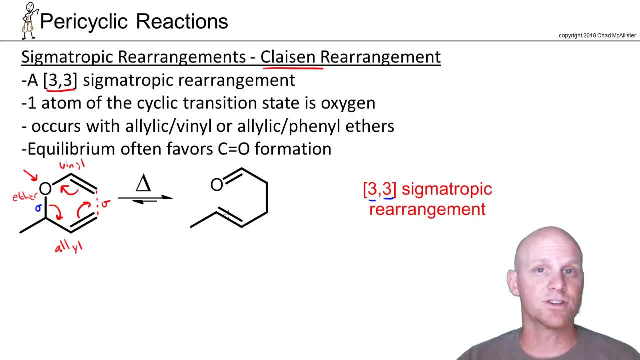 usually the keto form is favored just because the electrons are lower energy in a carbon-oxygen bond than in a carbon-carbon double bond. So that's usually what's governing the equilibrium here is just favoring formation of that carbon-oxygen double bond. 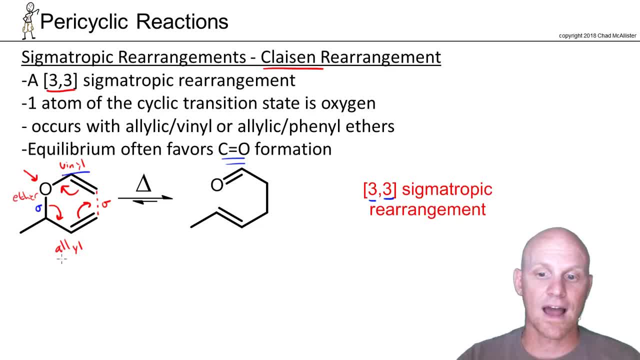 And again, how to recognize this. you've got a vinyl allyl ether. That's how you know. If it's not arranged for you, looking like it's almost forming a six-membered ring, then you should really redraw it till it looks like it is. 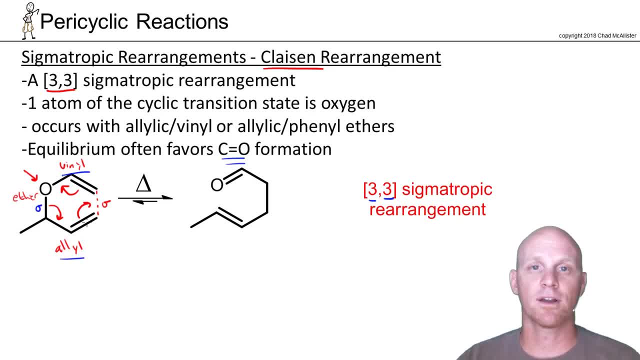 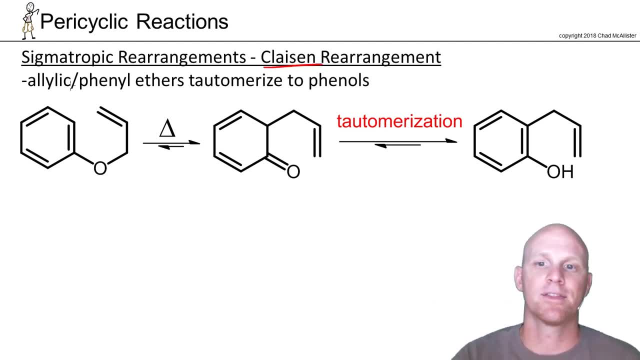 It'll be much easier to look at the the arrow pushing and predict what your product is going to look like. So we need to look at one special case for the Claisen rearrangement, and that is instead of having an allylic vinyl ether, you have an allylic phenyl ether. 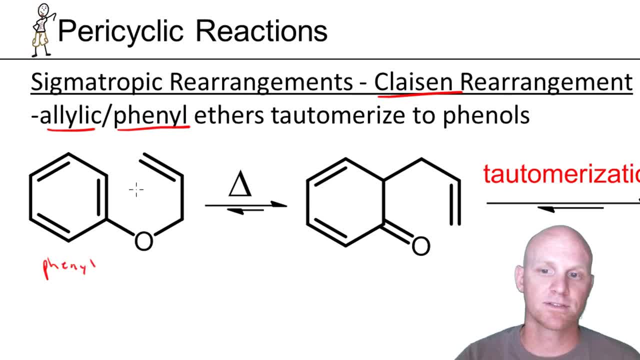 so a benzene ring here. So here's the phenyl part, here's the allylic part, And in this case your rearrangements can be just a little bit funky. But if again, look at the same cyclic movement of electrons here. so I'll move these here. 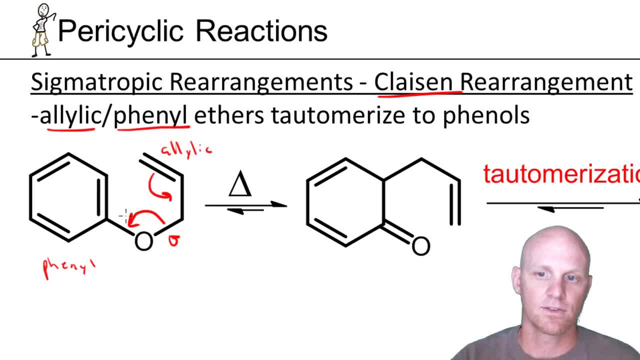 I'll move these here. That's where I'm breaking a sigma bond, and then we'll move these out here and that's where I'm forming a sigma bond, So where I'm forming and breaking 1,, 2,, 3,. 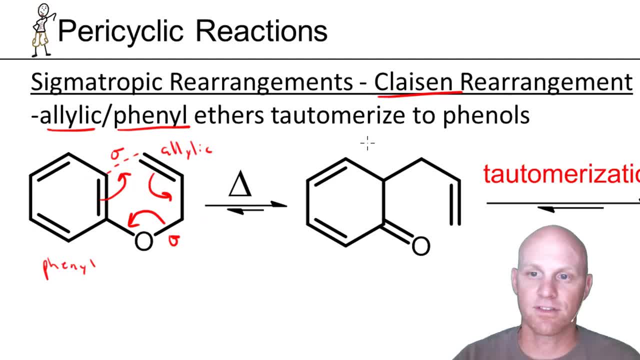 and on this side 1,, 2,, 3, and again that's what makes it a 3,, 3-sigma tropic rearrangement, just like all the Claisen's. But some things are going to be a little bit funky here. 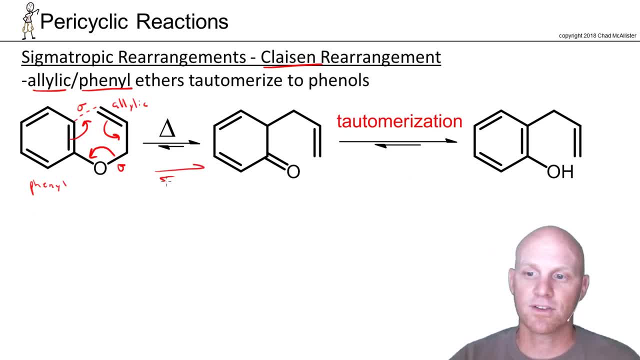 and again, the equilibrium here is going to favor formation of the carbon-oxygen bond, at least initially. but as you recall, with ketones there's always ketoenol tautomerization and most of the cases you've studied, the keto form is heavily favored. 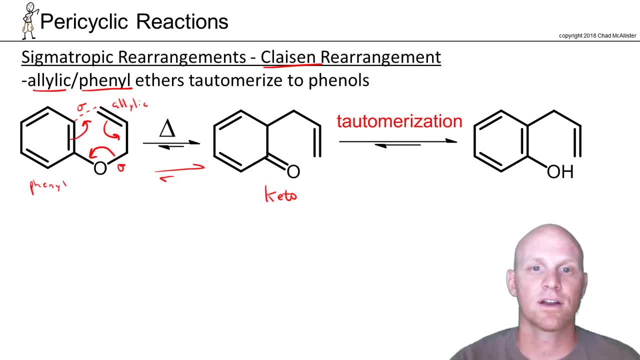 Well, that's not going to be the case here. so it turns out, if we tautomerize this, so notice, we're going to form a double bond here and make this just an alcohol, so and this would be essentially the enol version. 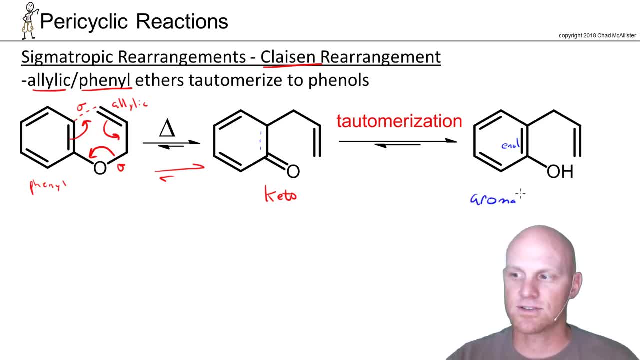 Well, there's something special about this enol version, and this enol version is aromatic. You've got a benzene ring right here and that makes it really stable, and so, as a result for Claisen rearrangement, starting with a phenylalanine,